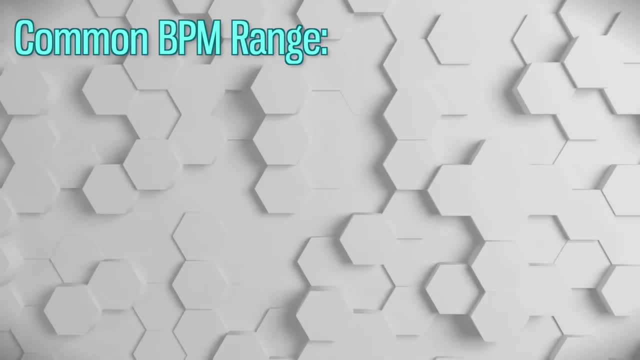 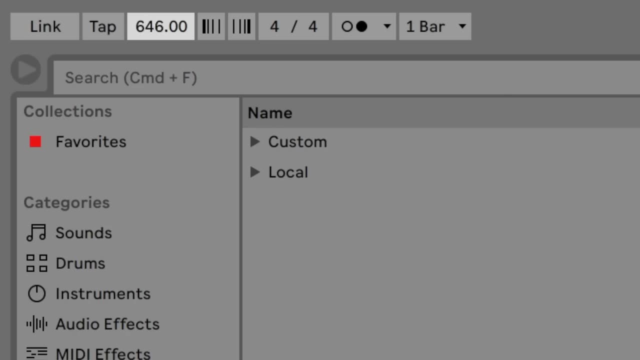 resulting in a faster song. Slower BPM makes for a slower song. Generally, you'll work with anywhere from 40 to 250 BPM. These numbers are completely arbitrary, but the point is you won't ever really have a need for anything outside that range. 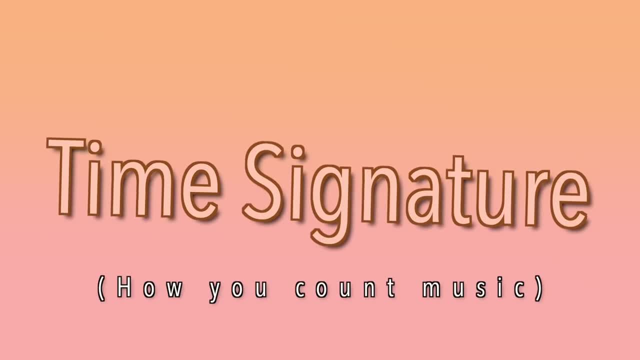 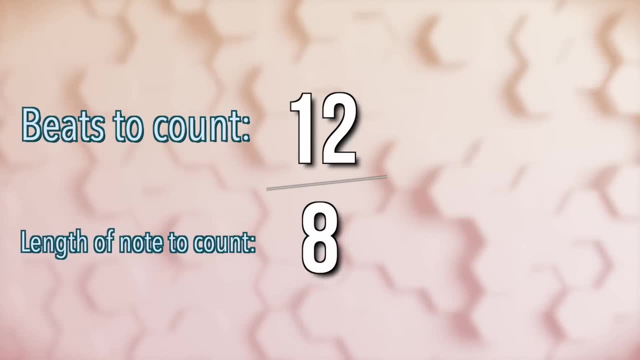 Time signatures expand upon this and determine how the music is to be counted. These are often written like fractions, with the top number representing how many beats will lie within a bar and the bottom number determining the length of note to count. The most common time signature. 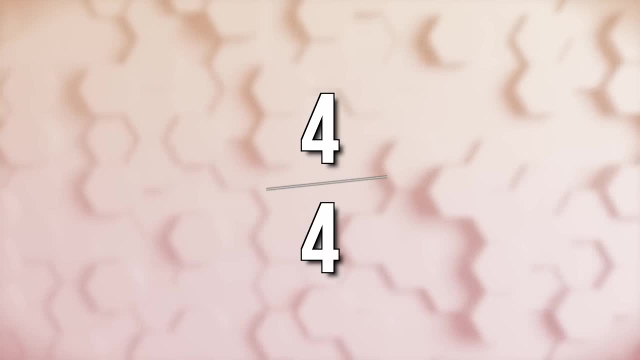 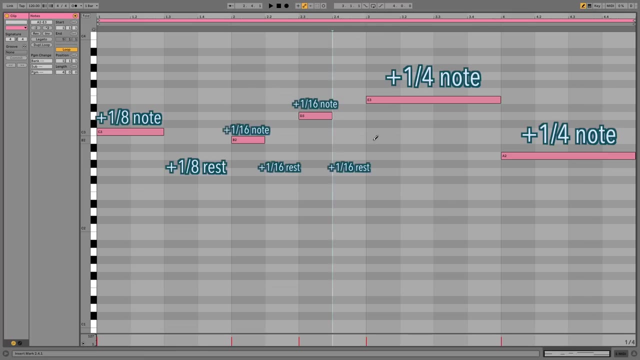 is 4-4. This means we count four beats in a bar and the length of notes within this bar must add up to the equivalent of four quarter notes. Granted, we can use any combination of notes and any combination of rests to fill up this space, as long as they add up to the equivalent. 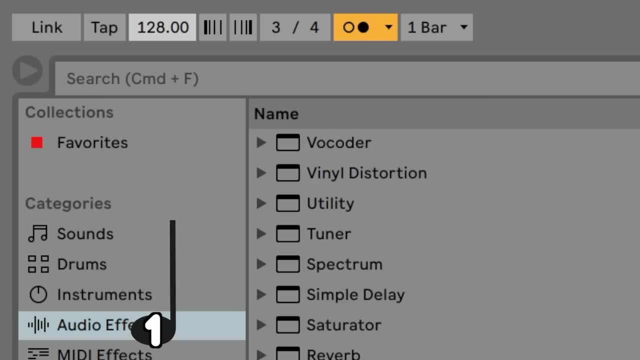 of four quarter notes Sound confusing? That's because it is. If we were in the time signature 3-4,, we would count three beats in a bar that are the length of three quarter notes. but if we were to double both of these numbers and use six-eight that, 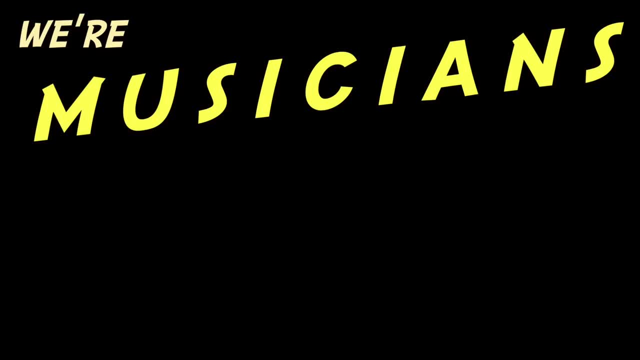 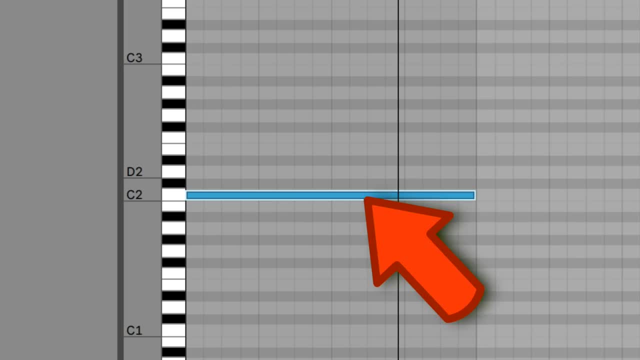 is actually different than 3-4, because, remember, we're musicians and not mathematicians. If any of this went over your head, just use 4-4.. Frequencies: This is a note. A note is comprised of a pitch and a duration. Pitch is the particular frequency. 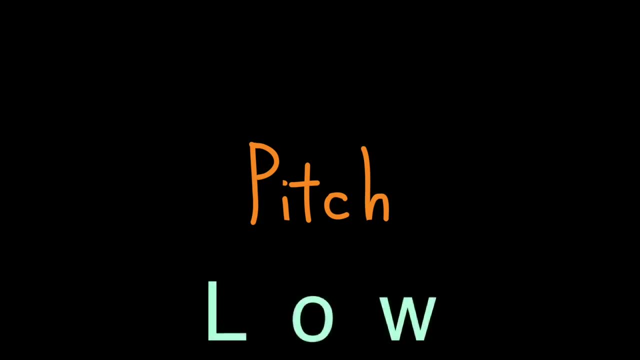 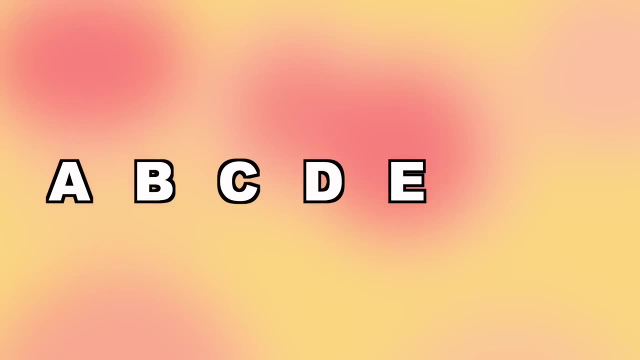 of a sound. measured in hertz, This determines how high or low a note is. Someone, somewhere, then decided to assign arbitrary names to pleasant sounding frequency values as the first seven letters of the alphabet: Any frequency value that is an exact multiple of one of these notes. 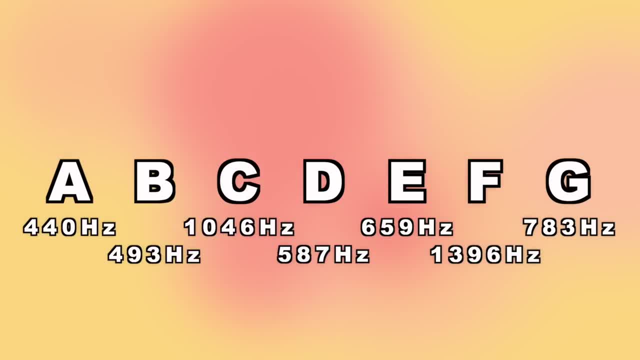 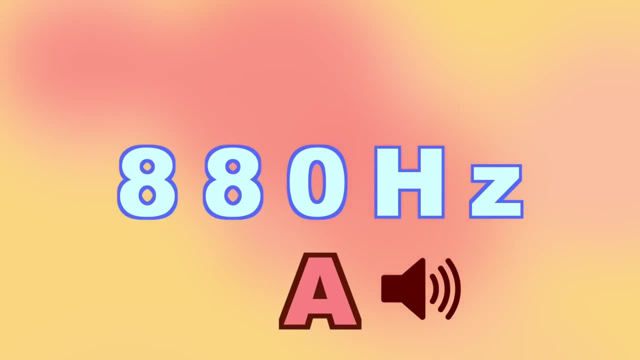 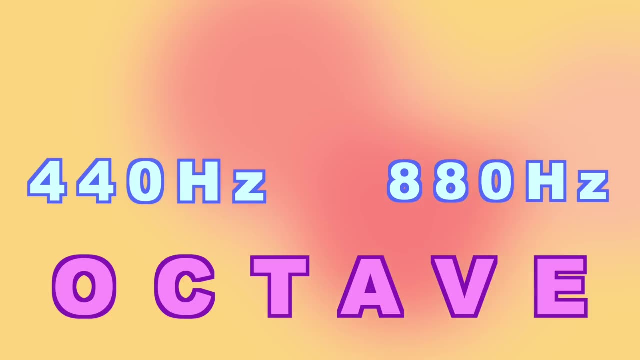 is also considered the same pitch, just played either slower or faster. For example, 440 hertz corresponds to the note A, But so does 880 hertz. since this is the same pitch, just played twice as fast, The gap between these two notes is called an octave, So to distinguish. 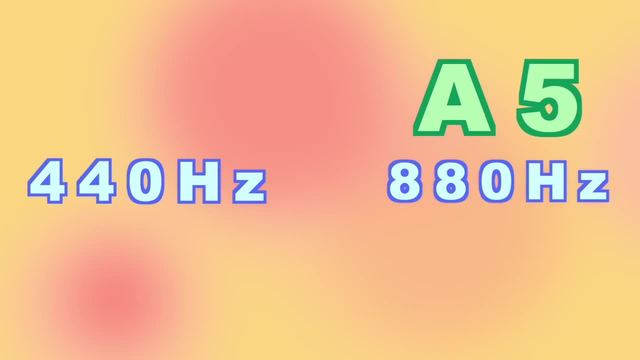 between these two notes. we often call them by their letter name and octave number. 440 hertz in this case is called A4, and is often used as the reference for tuning instruments Notes. A piano is a good way to visually represent notes, which is often why a piano roll is. 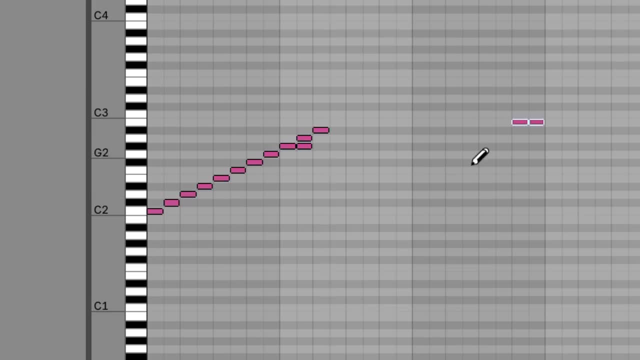 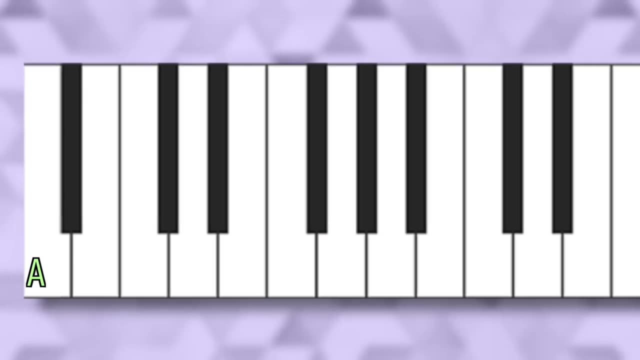 used in electronic music software as a way to draw in your notes even if a piano isn't the instrument you are playing. The lowest note on a standard 88-key piano is A0.. From there, every white note follows the pattern of B, C, D, E, F, G and then the next octaves. 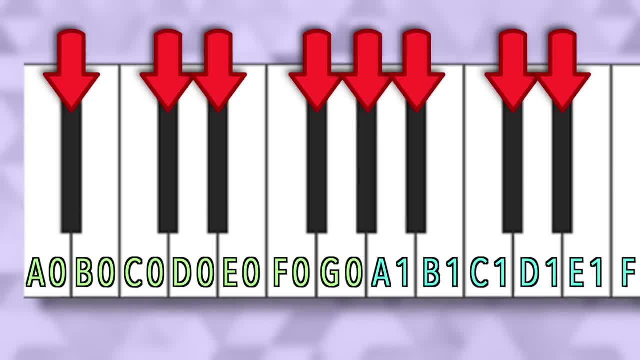 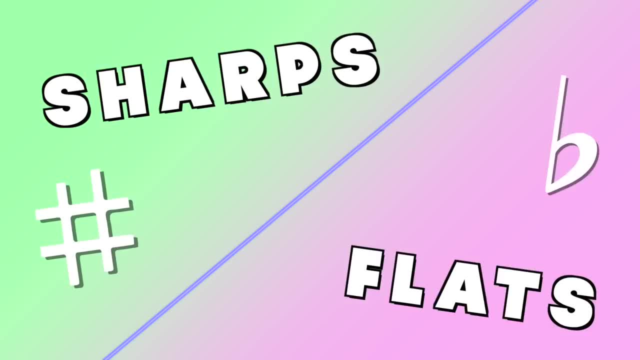 A repeating until the end. The black keys are named according to their location compared to the key, either to their left or right. To handle this, we use fancy terms called sharps and flats. Sharp means we go up to the next closest key and a flat means we go down to the next closest. 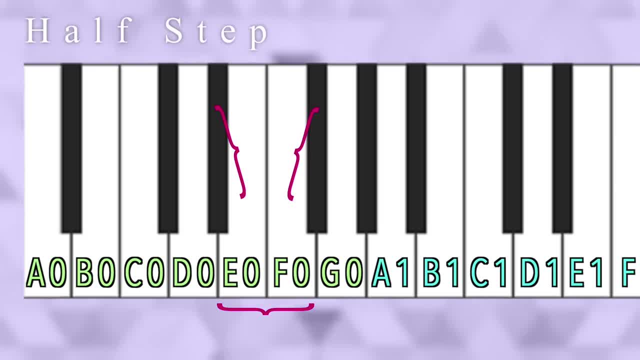 key. The gap between each key on a piano is called either a half-step or a semitone. For example, the black key directly to the right of C is one semitone above C and therefore called C sharp. However, as if this weren't confusing enough already, the same exact note is also called: 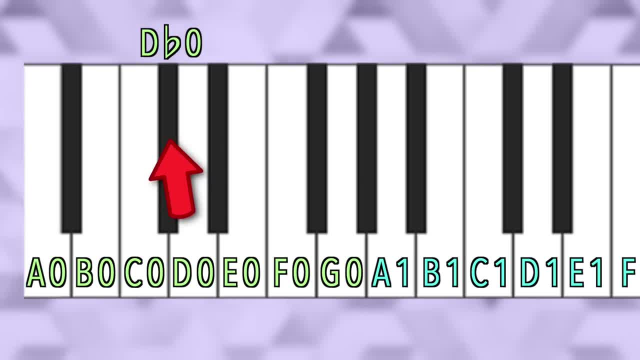 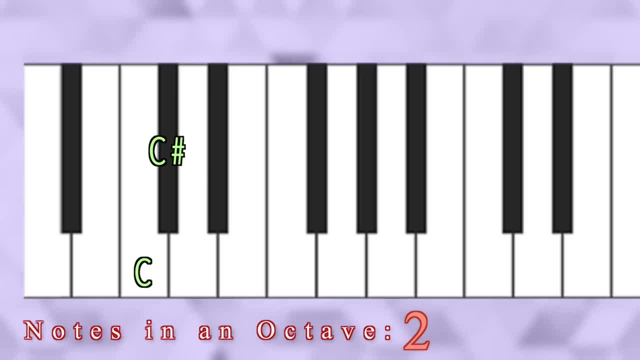 D flat because it lies one semitone below. So now to really hit it home, let's quickly recap all the notes in any given octave, starting with C, C sharp D, D, sharp E, F, F, sharp G, G, sharp A, A, sharp B, bringing us to 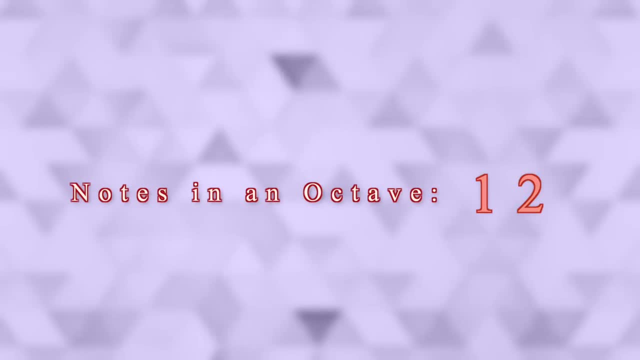 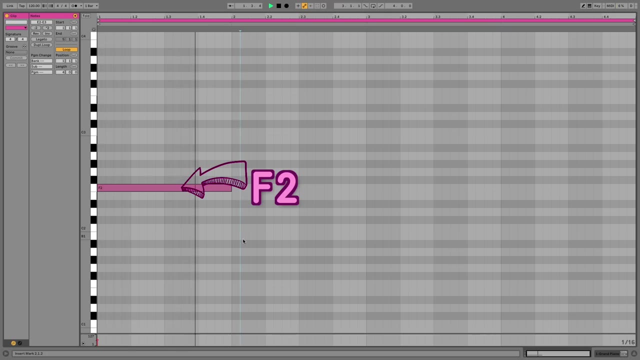 a grand total of 12 semitones in a single octave Scales are a collection of notes that sound good when played together. This note may sound fine by itself, but when played in succession with these other notes, it sounds like this: 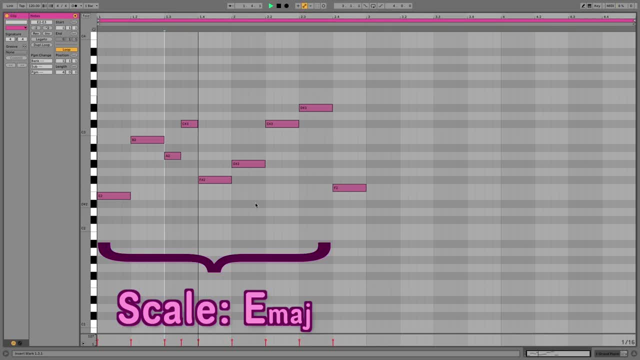 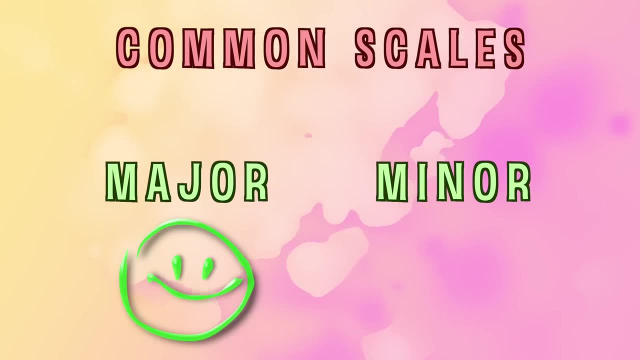 Not so much. This is because it's not in the same scale as the other notes and therefore is considered off-key. The two most common types of scales are major and minor. Major scales generally sound happy, while minor scales sound sad. A scale has a root note which it's named after. 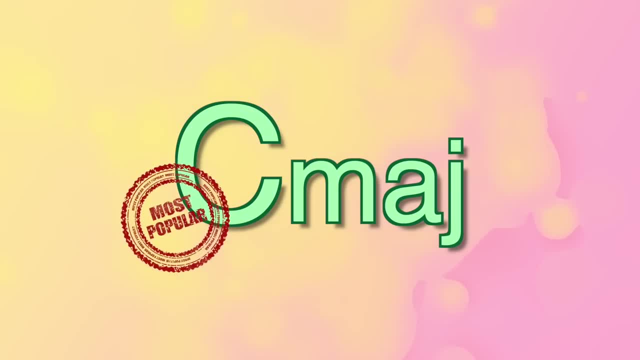 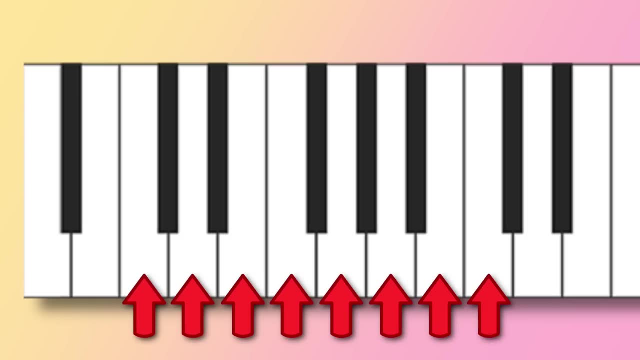 For example, C major. arguably the most popular scale is a major scale starting at C. This is popular because a C major scale uses only the white keys on the piano. You will recognize this as your Do Re Mi's. However, a major scale can be placed on any root note. 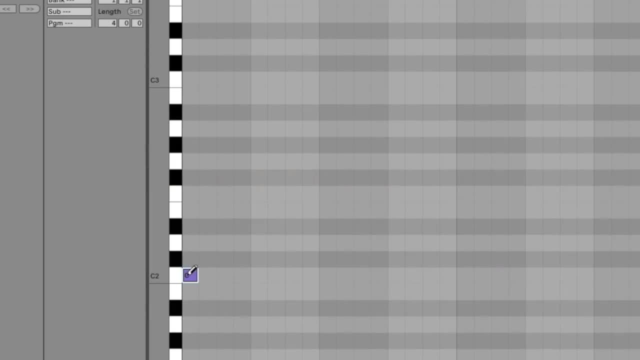 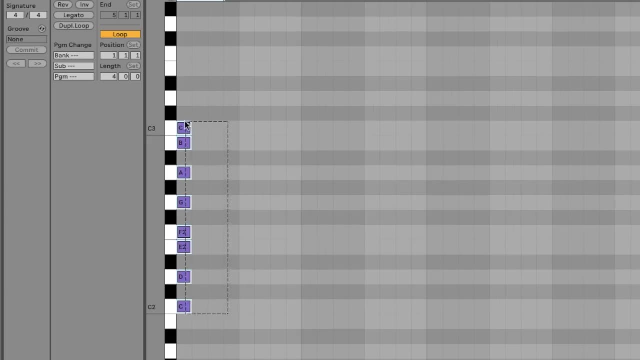 A nifty trick to quickly write any major scale is to draw in notes on all the white keys starting from C and ending at C. Then drag that to your desired root note. For example, this is a C major scale and now this is an E major scale. 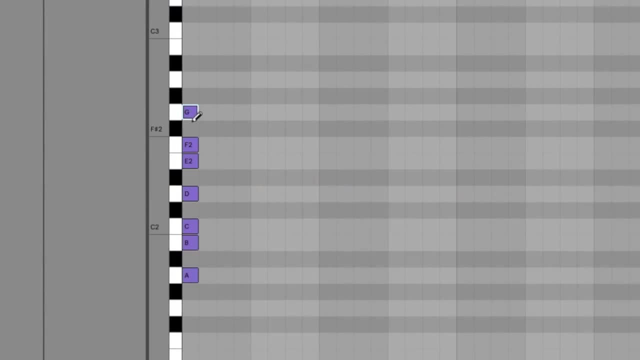 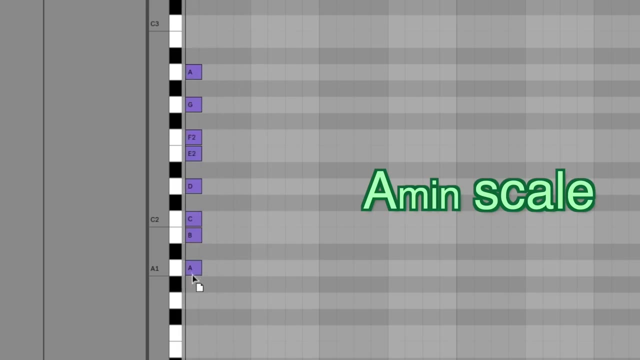 Similarly, writing a minor scale is as simple as drawing in all the notes on all the white keys, starting from A and ending at A, Then drag that to your desired root note. This is an A minor scale. Now this is a G minor scale. 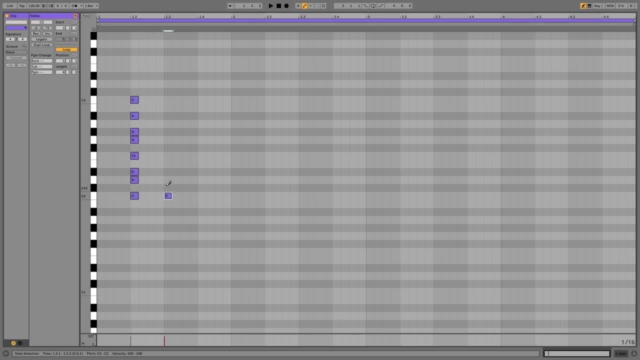 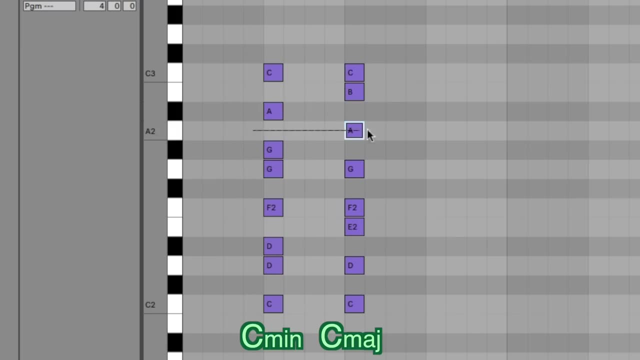 Your gut may be telling you that there's no difference between these two scales, since all I did was draw in the white notes, so they're the exact same. The crucial difference here is where I started. The gaps between the white notes will be offset depending on what note I started from. 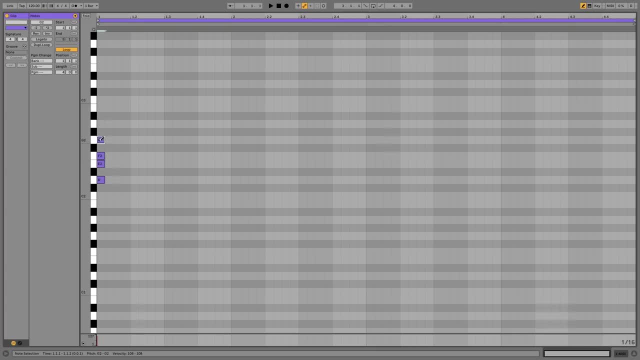 This process can be repeated for each root note. For example, drawing in all the white notes from D to D results in what's called a Dorian scale, But if you're just starting off, I'd recommend sticking with only major and minor scales. 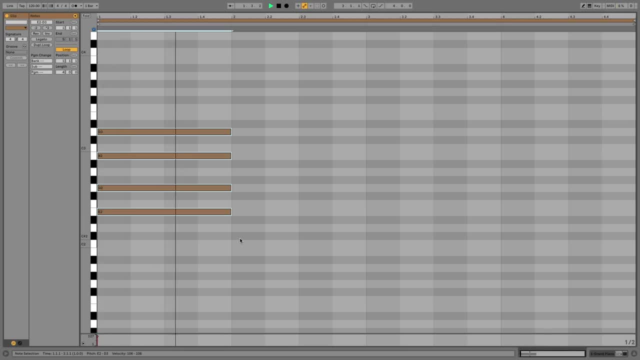 for now, Chords. Chords are multiple notes played in harmony at the same time. The most common type of chord consists of three notes and therefore is called a triad. A chord is named after its root note and its quality. For example, this is a C major chord. 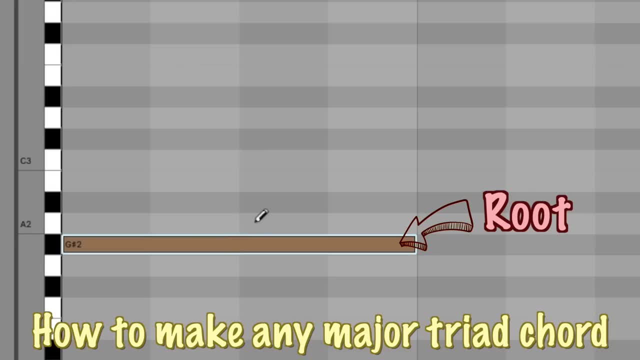 An easy way to remember how to make major chords is to pick your root note and draw in another note four semitones above that, and then finally one more three semitones above that note, or a total of seven above your root. 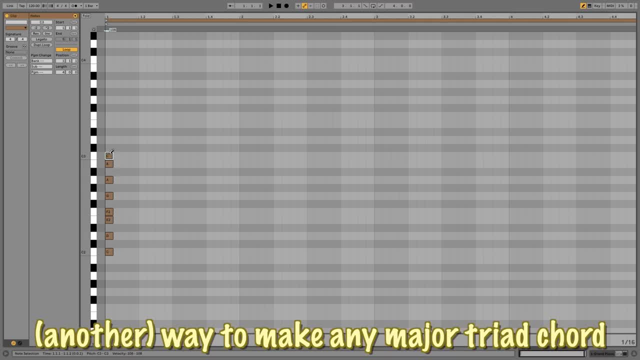 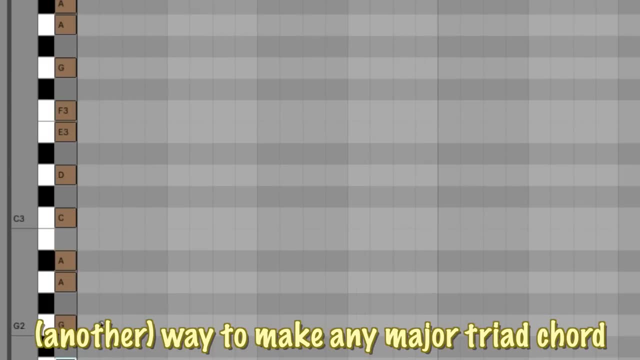 Another, even quicker way to remember major triads is to draw in a major scale using the trick previously described. let's pretend I want to be in F major. Now pick any note to be the root of my chord. let's say A sharp. 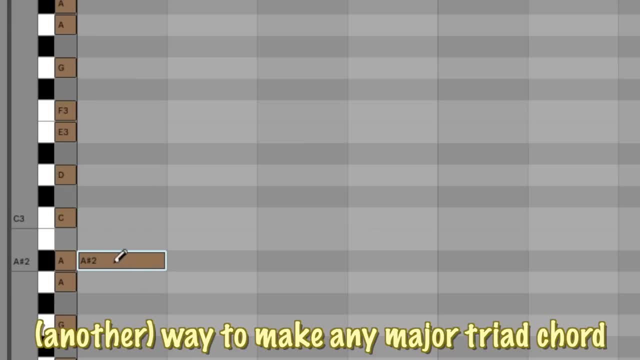 From here, draw in a note at every other key in this scale moving upwards. In this case, we skip over C, the next highest note in the F major scale. draw in a note at D, skip over E and draw in a note at F. 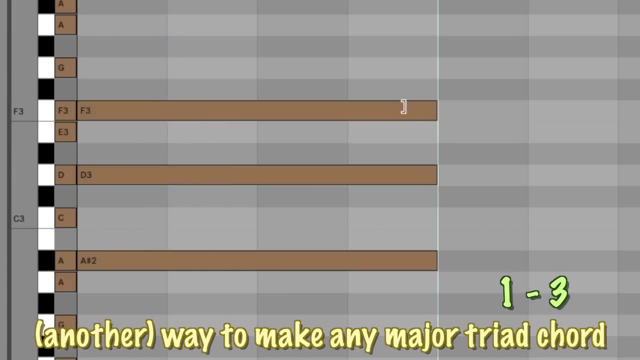 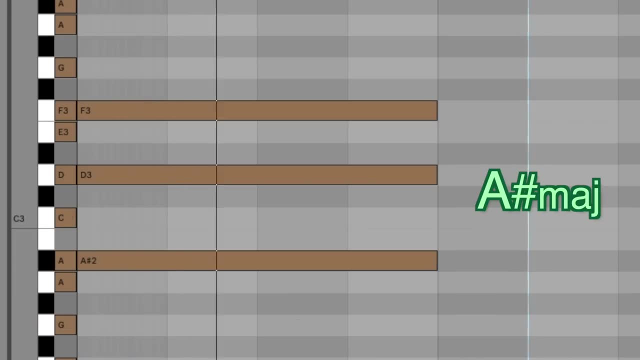 For this reason the major chord is referred to having the pattern of 1-3-5,. since our root is the first note and from here we use the third and fifth note to draw in a B minor chord, We now have an A sharp major chord. 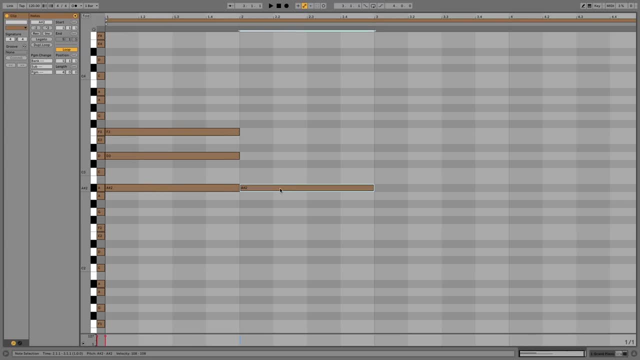 And, just like magic, it also follows the pattern we previously described, where the gap between the root and the second note is four semitones and the gap between the root and the third is seven. And making minor triad chords is also very similar. 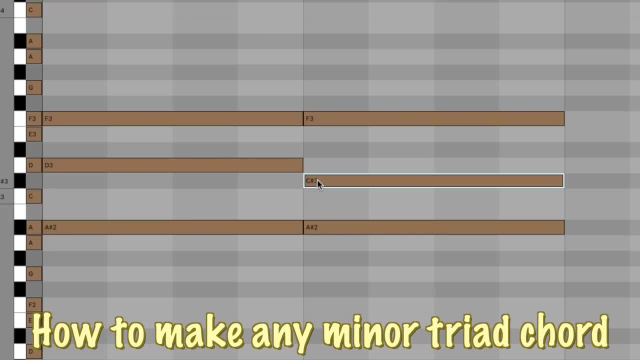 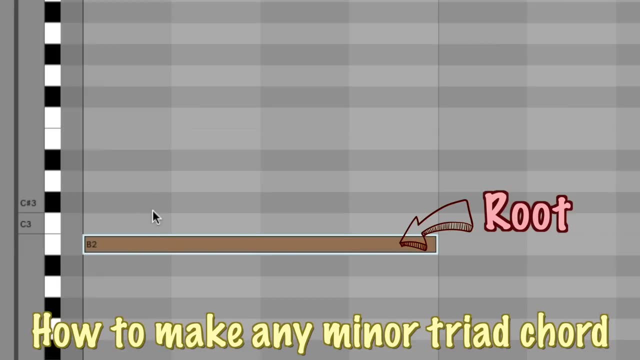 In fact the only difference from a major triad is you drop the second note down by one semitone. So to make a B minor chord, for example, draw in your root note at B, move up by three semitones again, rather than four in a major chord, and then your third note, four semitones. 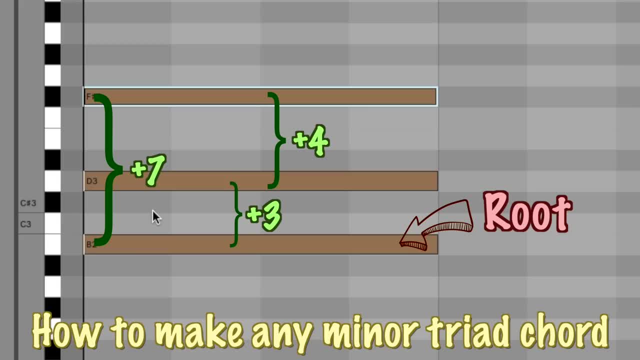 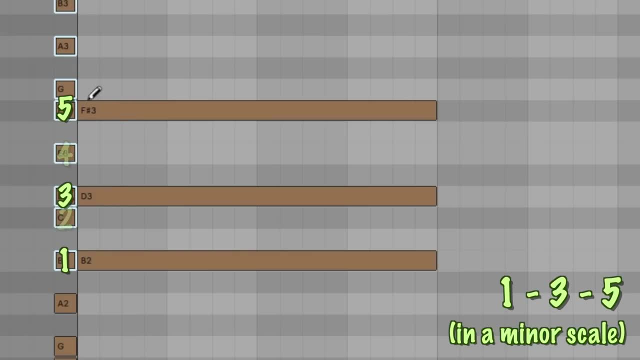 above that, Again, this is still a total of seven semitones above your root. From here we have a B minor chord And, yes, this is still the 1-3-5 pattern if you're in a minor scale.